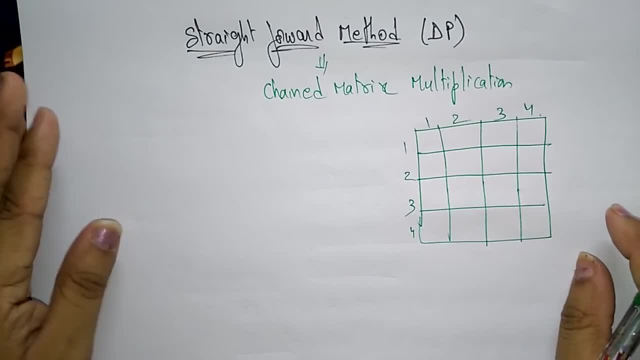 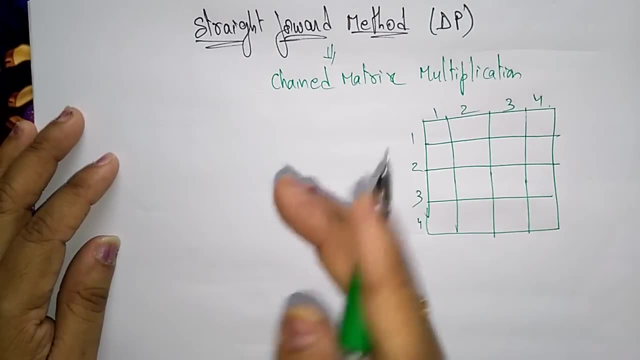 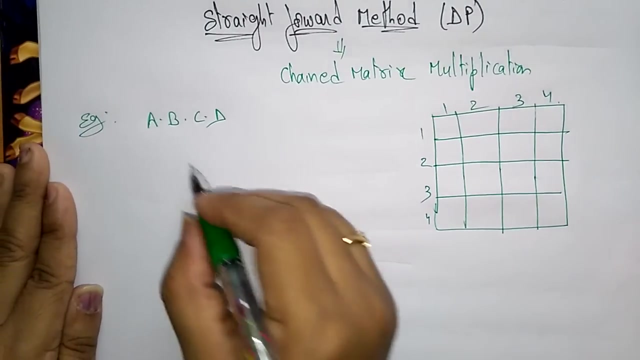 help of the tabulation method we can fall the chain, matrix multiplication. so here a cost of a is zero. uh, first we have to take uh, i said a dot b, dot c, dot d. let me take the example. okay, so, each having the size, what are the sizes of a and b, what i have taken? the previous example, 13 by 5. 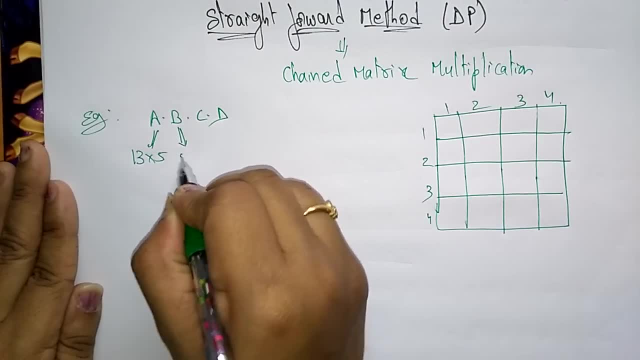 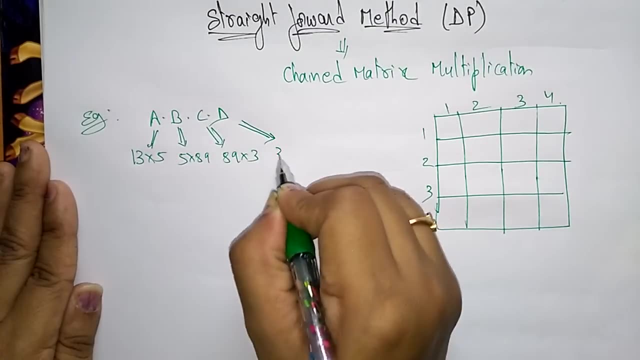 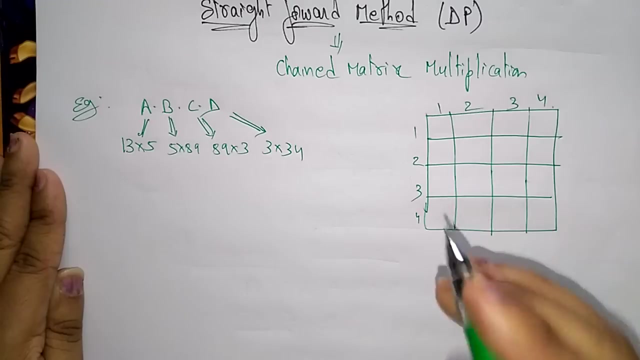 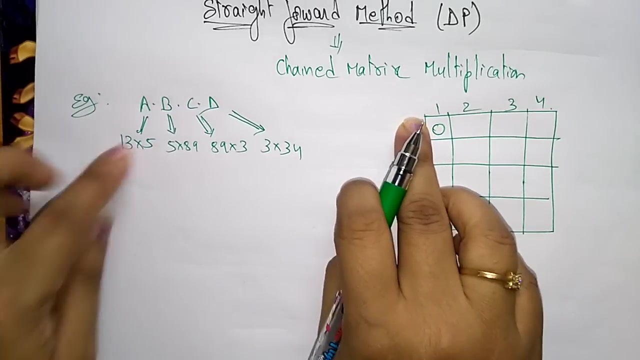 so this is 13 by 5 and b is 5 by 89, c is 89 by 3 and d is 3 by 34. so these are the sizes of the matrix. so first, the cost of a is 0 because it does not multiply without any value. so one one uh cost of a itself. 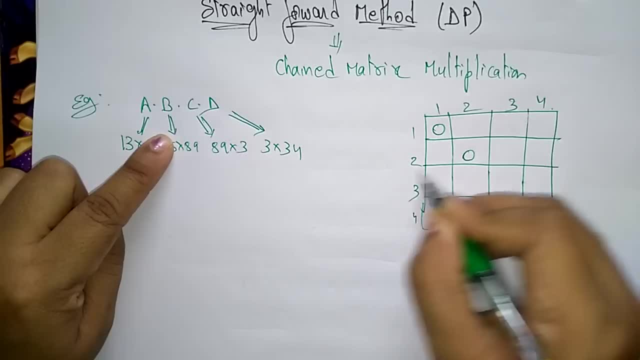 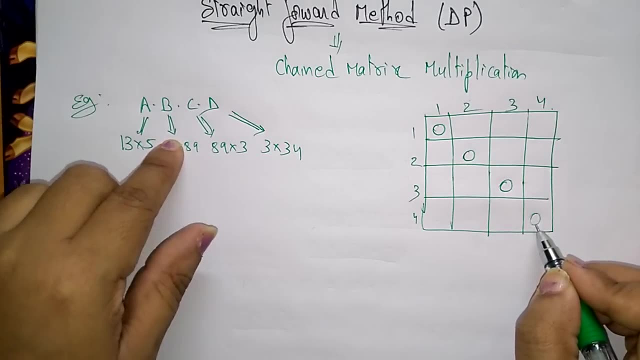 is 0. in the same way, the cost of 2 by 2 matrix, that is second row in the second column, the cost of b is 0 and c is 0 and the d is 0 because, uh, it does not multiply without with any value. i means it does not multiply with any value. 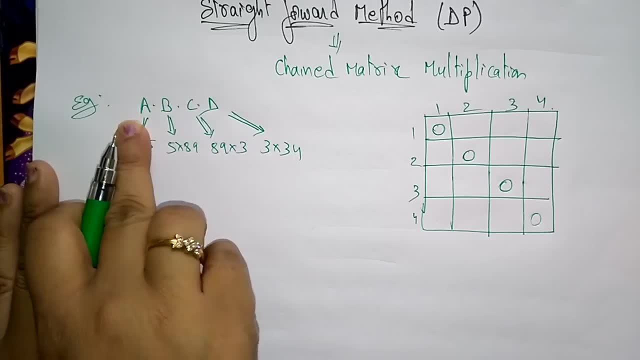 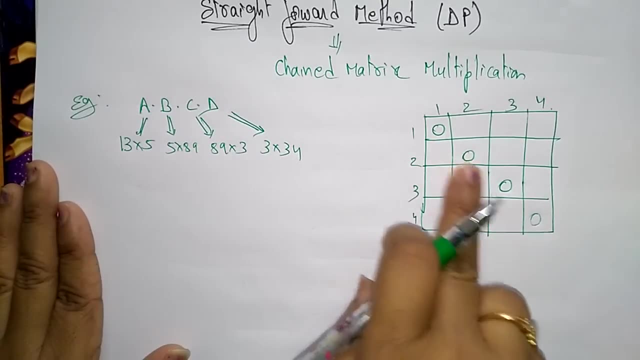 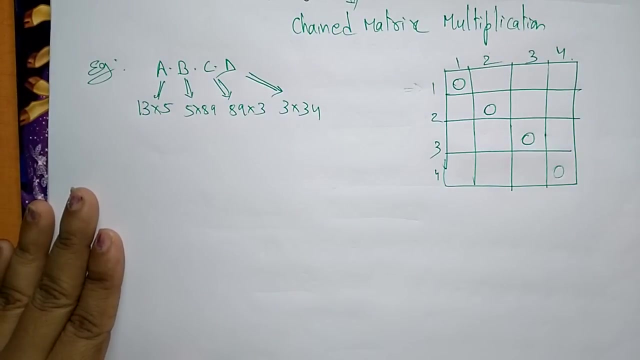 a cannot multiply with a, b cannot multiply with b, because we have to multiply a into b, or b into c, or c into d or a into c, like that. a into a is no, not there, so that's why we are keeping all zeros here. okay, so now let's take the first sequence. so here the first sequence. so in this first sequence, 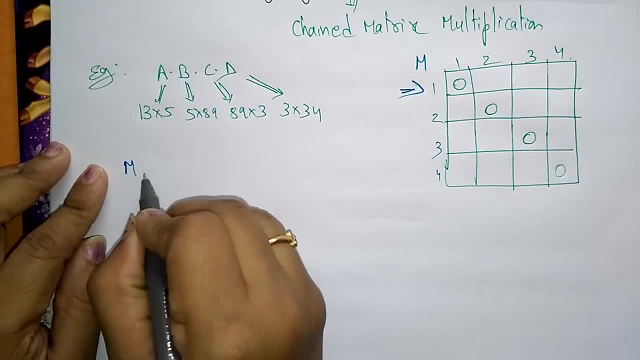 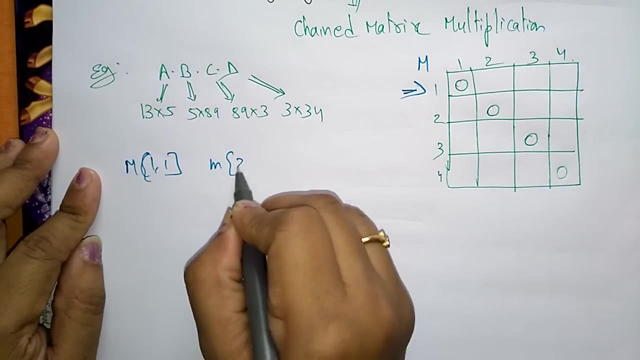 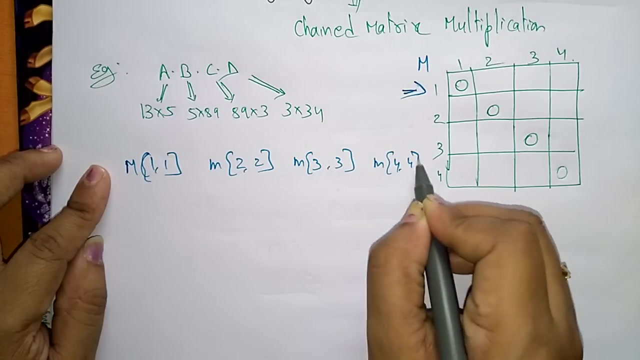 let me take the first sequence. so it is the size of the matrix. represent m m of 1 by 1, m of 2 by 2, m of 3 by 3 m of 4 by 4. so here this is the a, b, c, d. so these are. 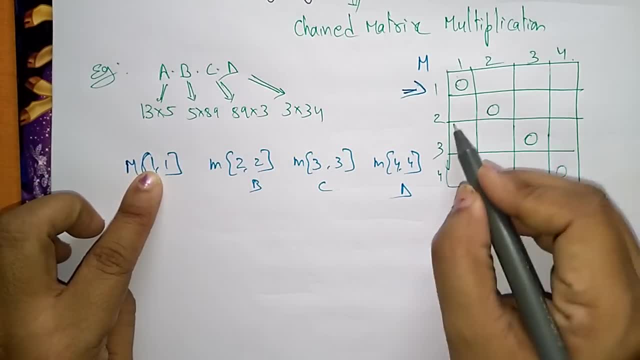 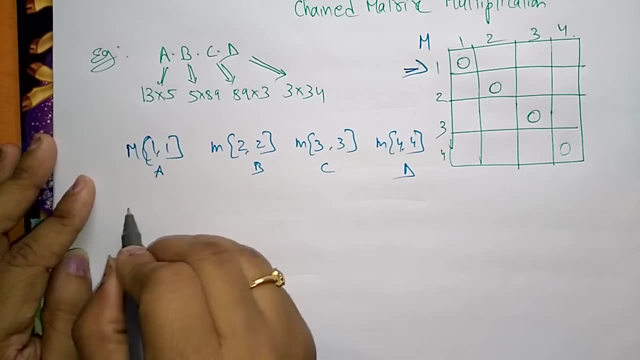 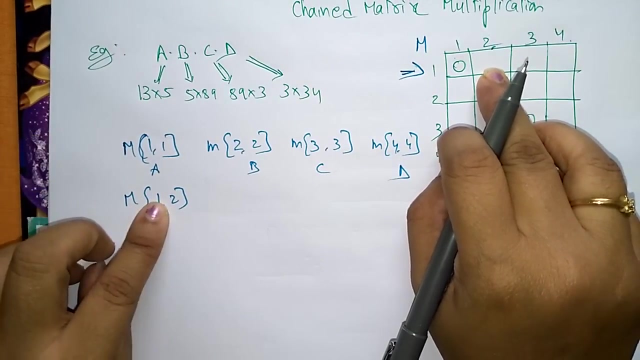 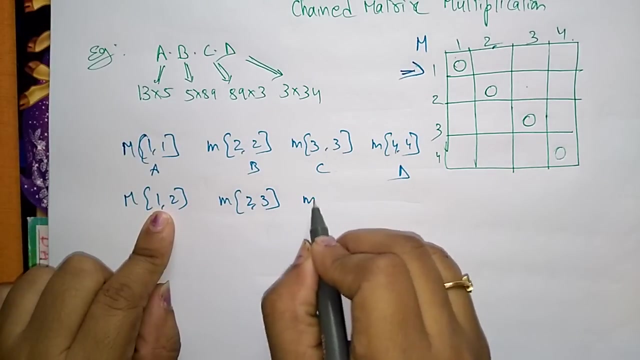 all small sub problems. so let's say these are all the small sub problems and these sub problems are 0. first and next. multiply two matrices, so that is m of 1 comma 2. so this is this: we have to find out the value for this: m of 1 comma 2, m of next, 2 comma 3, m of 3 comma 4 means just multiplying two matrices. 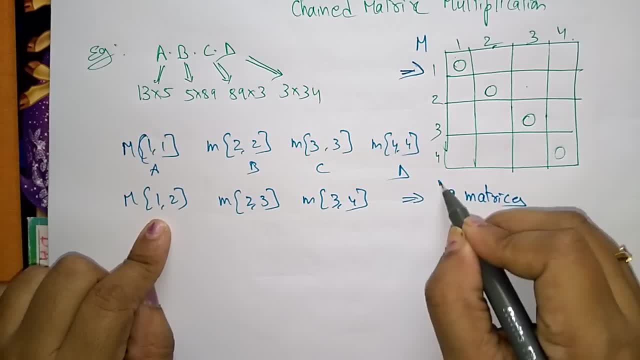 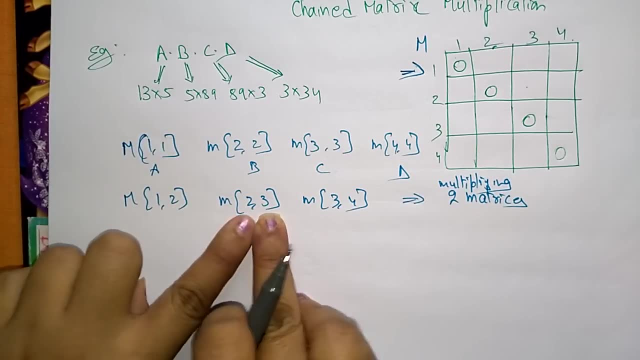 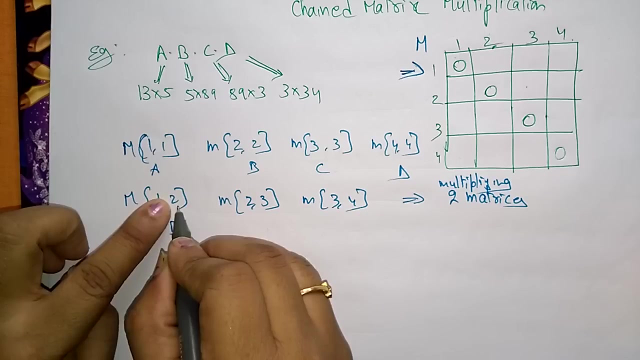 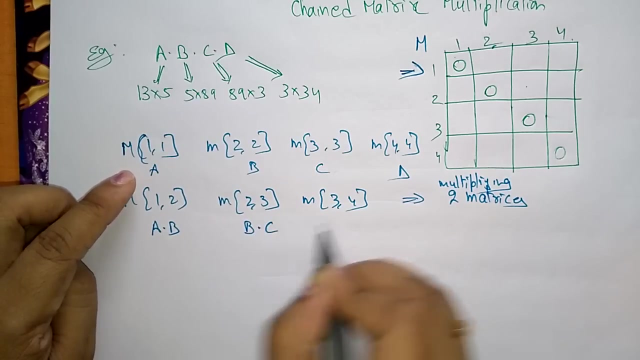 multiplying two matrices. so here 1, 2, 2, 3, 3, 4, like that. so 1, 2 means a dot b, 1 is a, 2 is b, and here 2 means b, b, dot c and 3 means c and 4 means d. so we have to find out the value of a dot b. 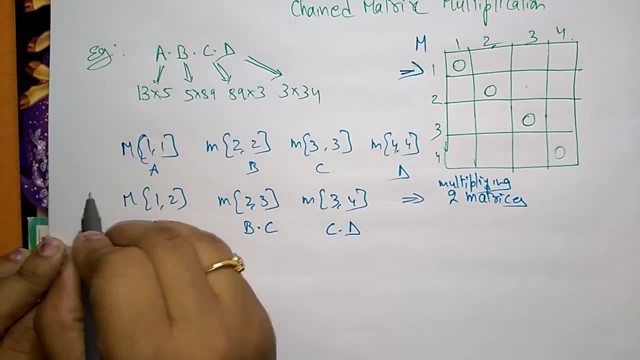 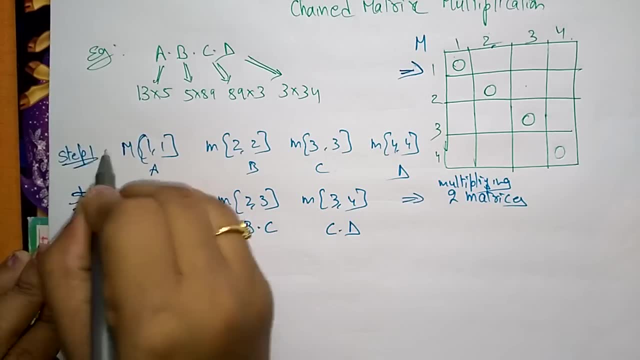 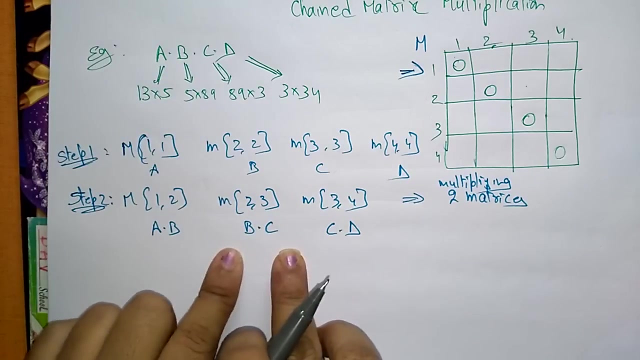 b dot c. c. dot means just first. first i am doing only the. this is step one, step two. so here i am just multiplying two matrices. okay, the final. i have to multiply four matrices. first i am multiplying two matrices: a dot, b, b dot, c, c dot d. so what is the values for this? let us see. 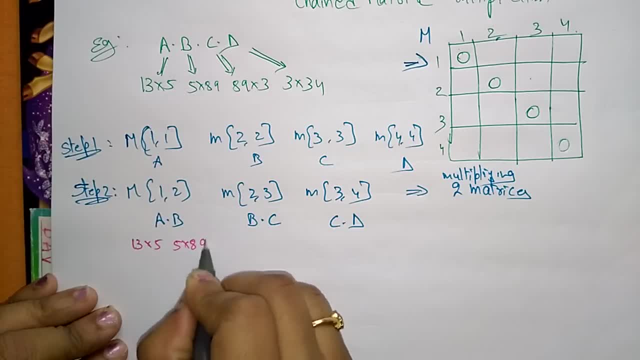 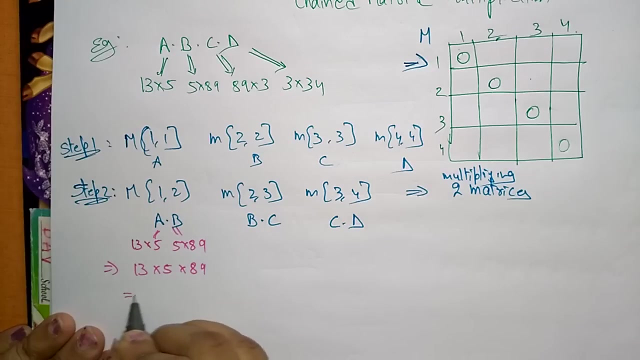 so that is 13 by 5, 5 by 8, 9. so from this we have to multiply 13 into 5 into 89, so this is the size of the matrices. so from this we have to take 13 into 5 into 89, so the result is 5785. okay, so just. 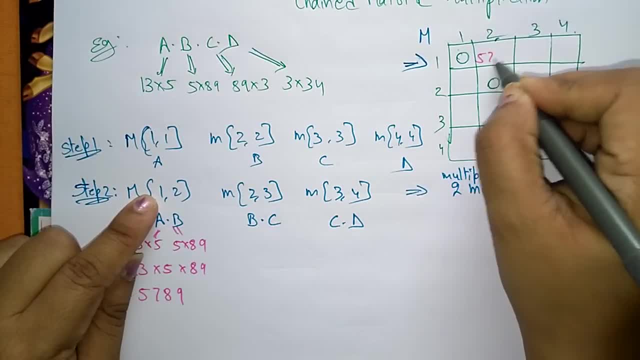 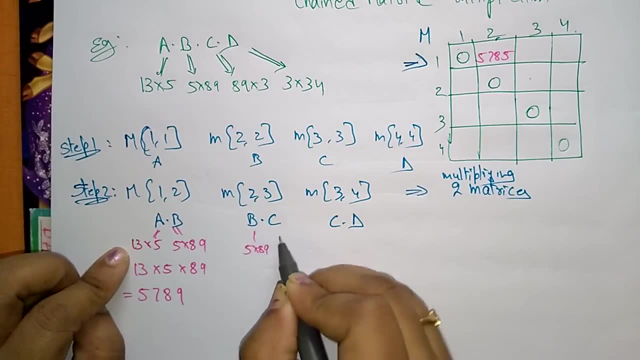 write m of 1, 2 is fifty hoped and miss is 5785, now bc. so what is the size of b? 5 by 89 and c is 89 by 3.. so from this 5 into just write 189 and three, the result for this is: 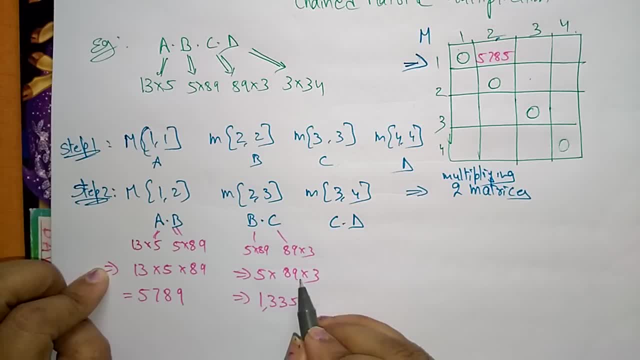 3. 배 a 2.5这是 1003x8ivalence3and4- 335.. So when you multiply 5 into 89 and 89 into 3, you will get 1335.. So I already calculated, so that's why I am directly writing the number here. So that is size of 2 of 3, second row and the third. 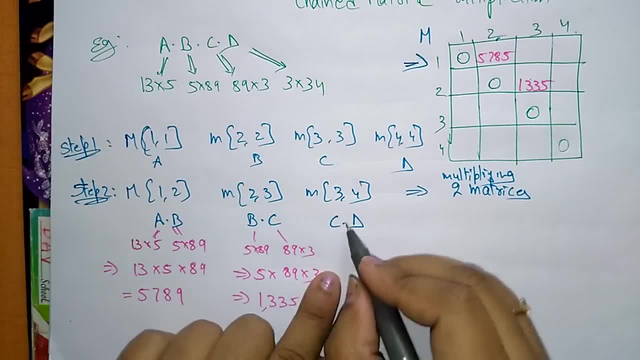 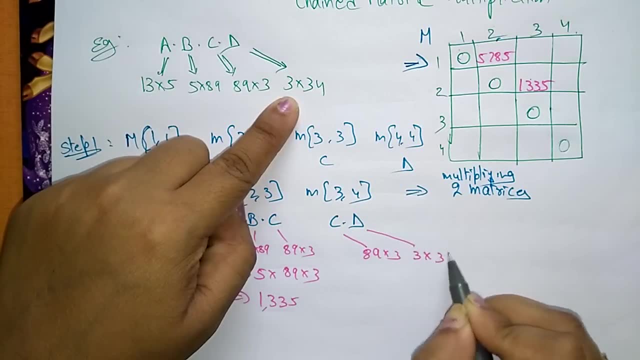 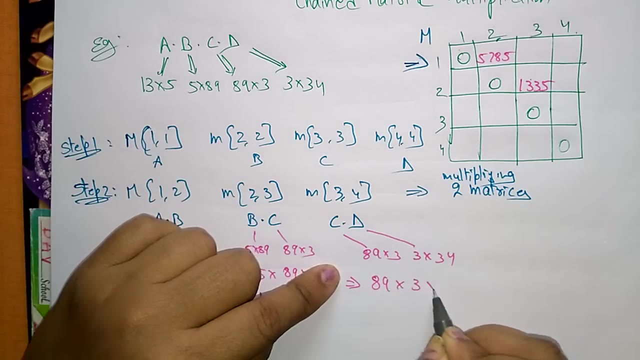 column, that is 1335.. And coming to C, the size of C is 89 by 3 and size of D is 3 by 34.. So from this 2 we have to take in this 2, we have to take only one value: 89 into 3, into 34.. So the result: 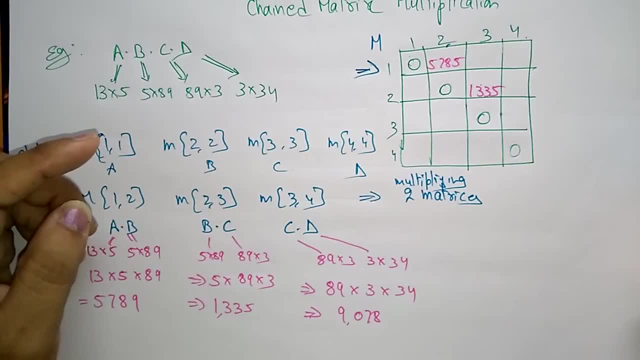 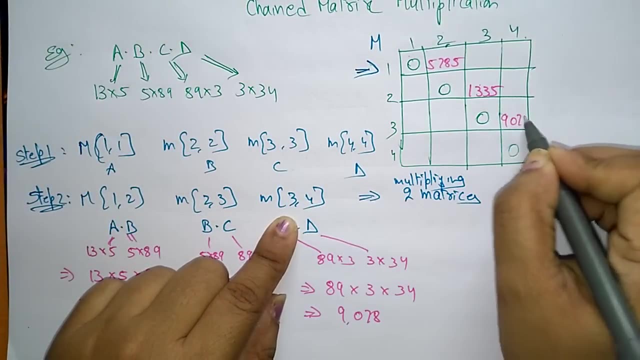 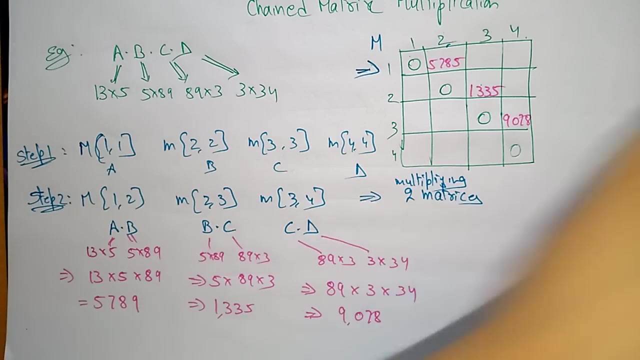 of this is 9078.. Okay, so that is 3- 4.. The 3- 4 size is 9078.. So the multiplication of 2 size matrix is over. Now let us take the 3 matrices The size of we have to multiply. 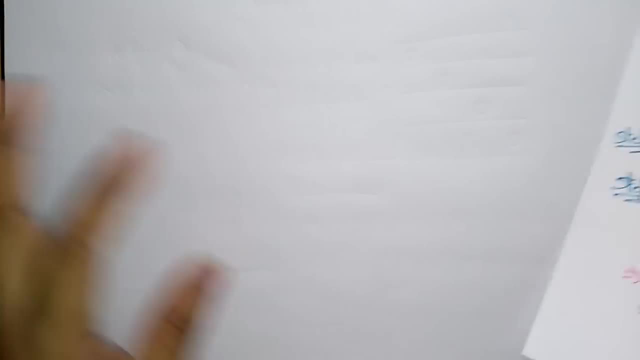 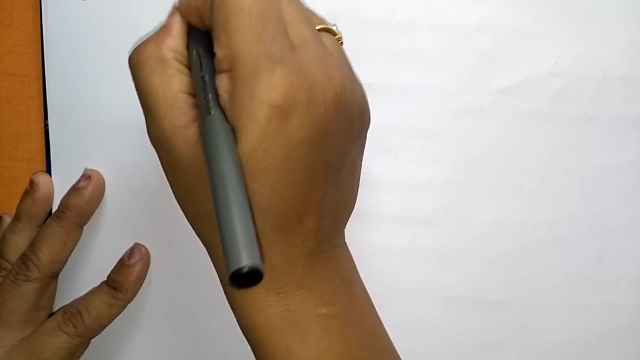 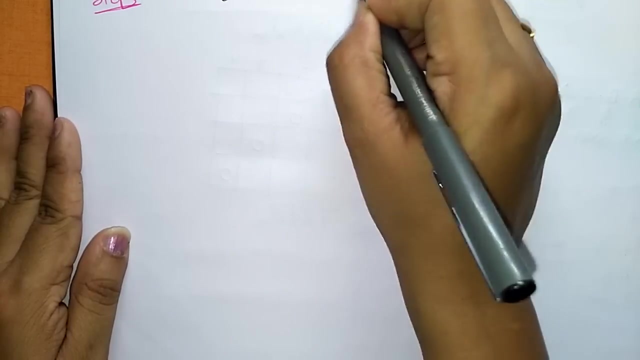 1, 2, 3, 4. 3 matrix. Let me take: So 1: 1 is over, 1, 2 is over. Now take 1, 3.. So next step, Step 3. M of 1, 3.. So what is the possibilities of 1, 3?? So there are 2 possibilities for this. 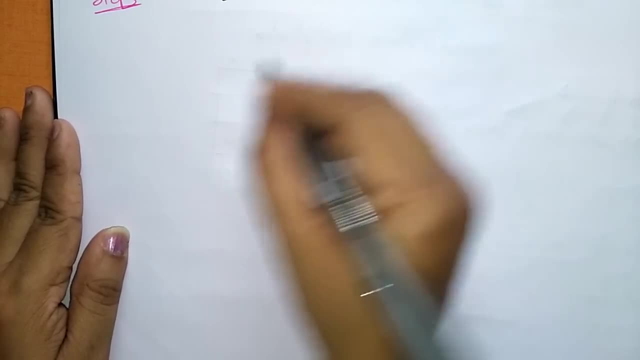 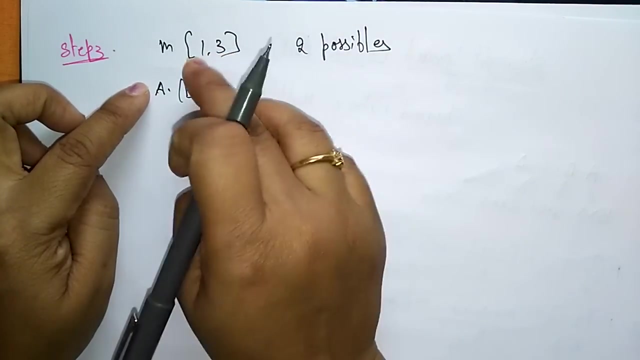 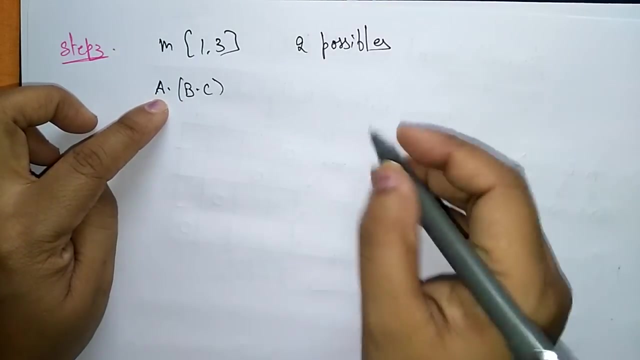 multiplication. The 2 possibles are there, That is a dot b, dot c. So if you want 1 into 3. First you have to take 1 to 3. You have to in the middle. that 2 element is there. So a dot b, dot c or 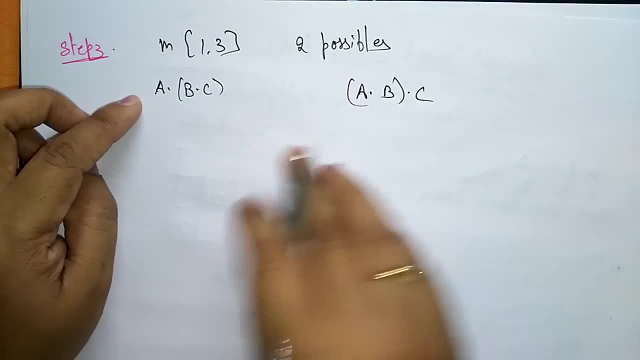 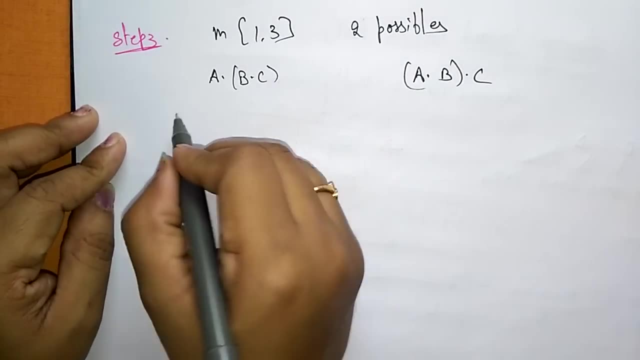 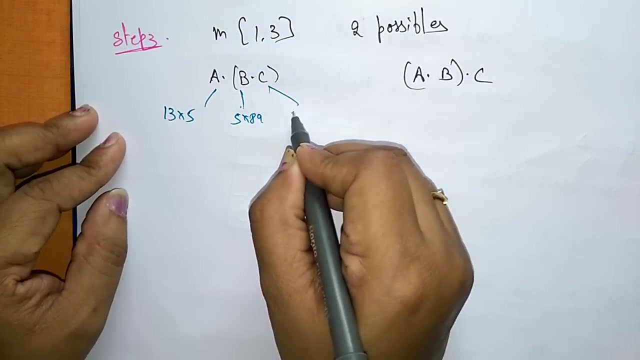 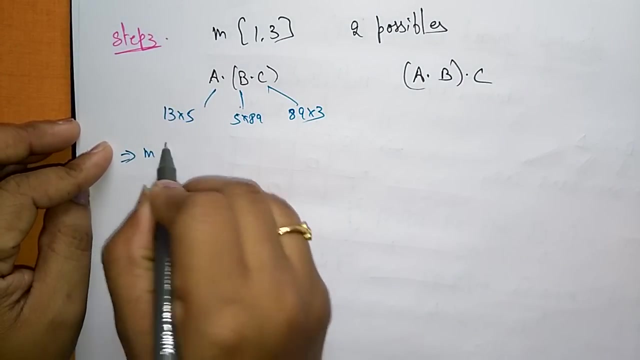 a, dot b, dot c. So for this multiplication there are 2 possible ways, So let me write those. So a is 13 by 5.. b is 5 by 89.. And c is 89 by 3.. Okay, 13 by 5.. It's nothing but m of 1 comma 1.. 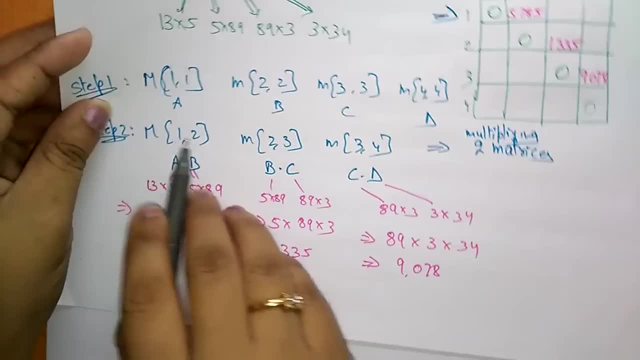 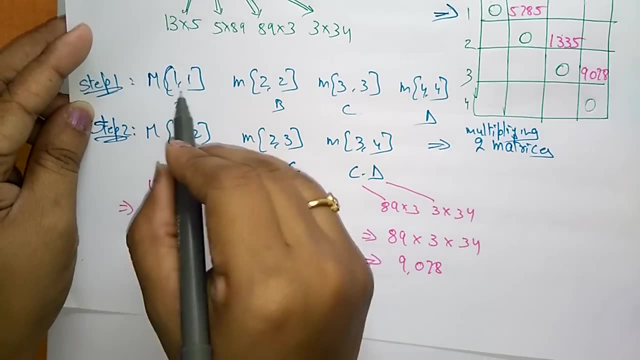 So why I have written 1 comma 1.. So 13 by 5. That is a a is 1 comma 1.. 13 by 5 means a a is 1 comma 1. So that I have written. 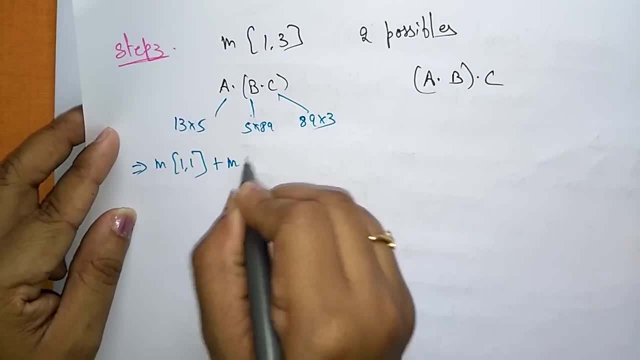 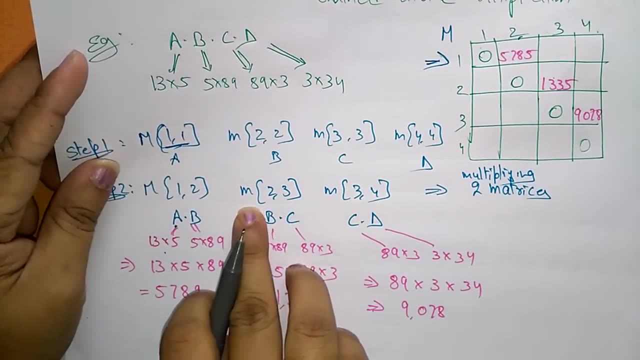 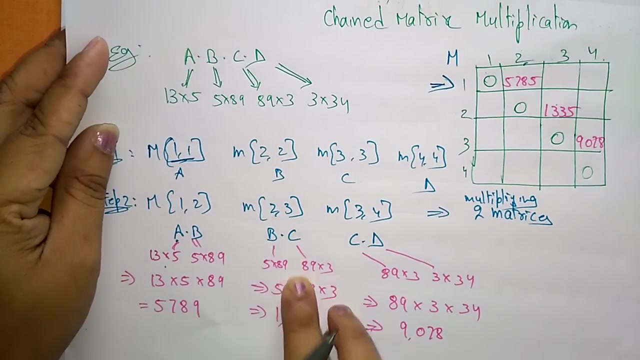 mof2,3.. mF ofс comma n and a, 0 comma 1P plus M of2 comma 3.. b means So: here next r one of a and b2 comma 3.. So b2 comma 3.. I have written around How to dolegen. 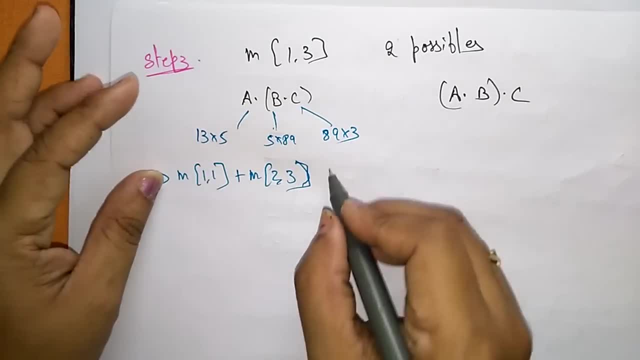 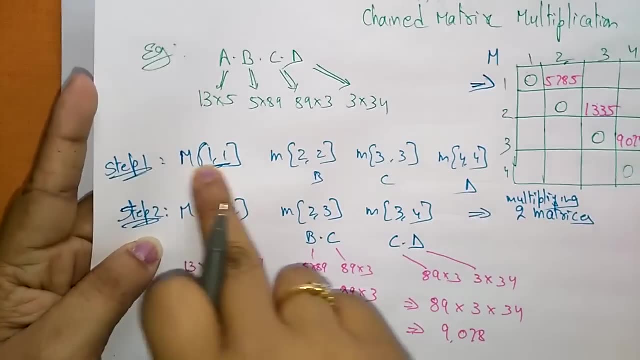 Next esp And p plus Plus. It means just b- C. Don't be confused. f 1- a is right here, and then c, a is nothing. but When you have these two possibilities to subtract m of 1.. 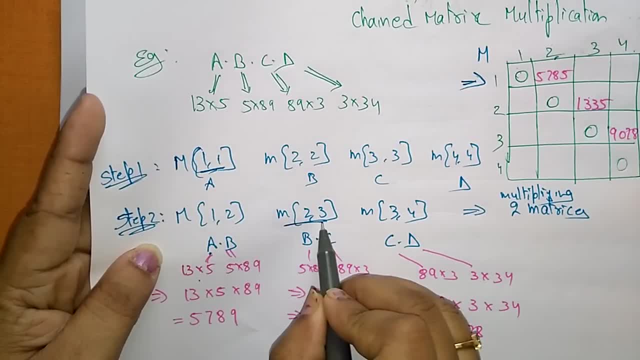 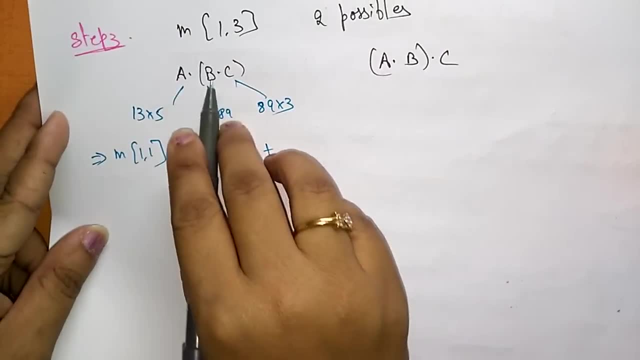 of 1 comma 1, and b dot c is 2 dot m of 2, 3. already i have taken multiplied b dot c means m of 2, 3, so that i have written: b dot c means m of 2, 3 plus. this multiplication is over and this 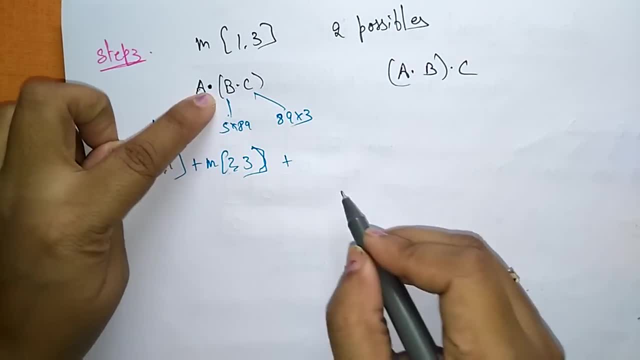 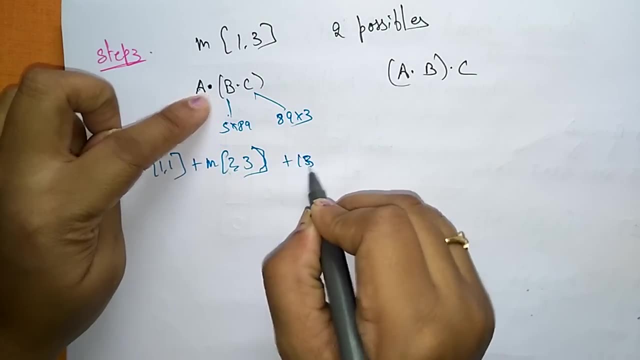 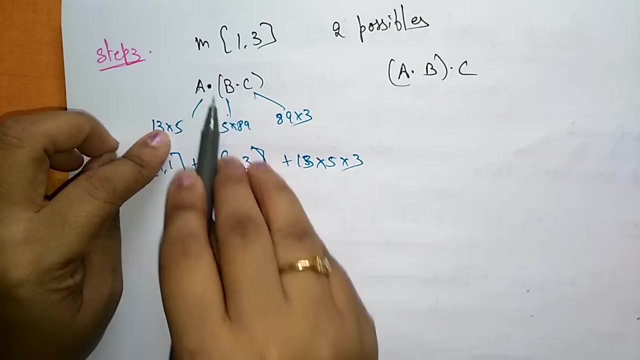 multiplication is over. now i have to calculate this dot, the cost of this dot. okay, so the cost of this dot is 13 by 5, by 3, so the cost of a is 13 by 5. so dot b, dot c is already 5, is there. 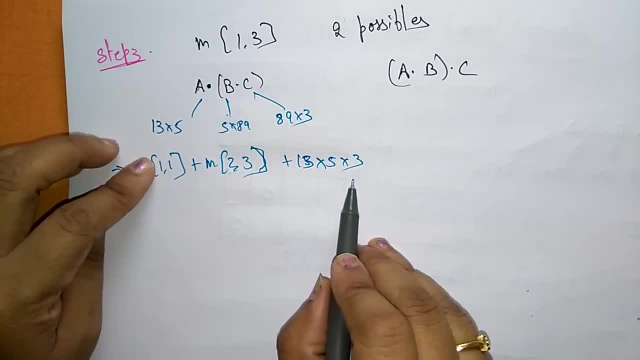 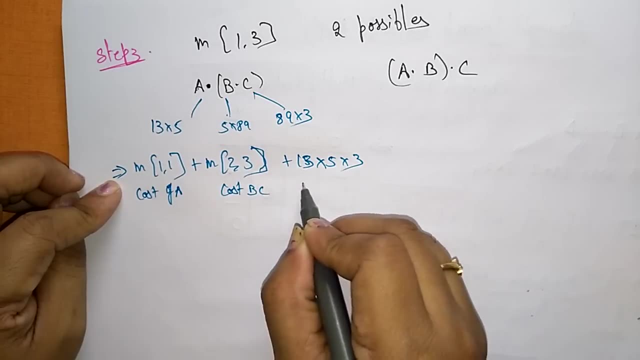 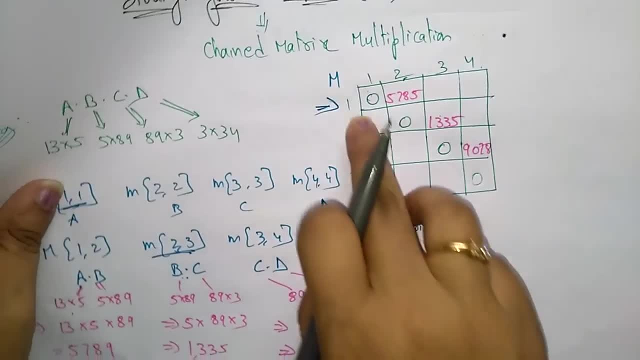 so this is the dot matrix size. so this is the dot matrix size. so this is the dot matrix size. so for this m of 1 comma 1, what is the value of m of 1 comma 1, 0? so just write 0 plus m of 2 comma 3. 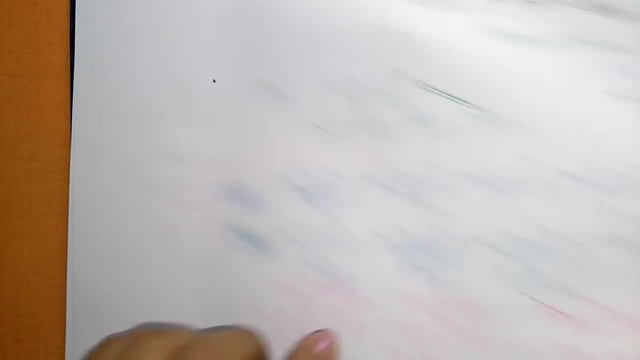 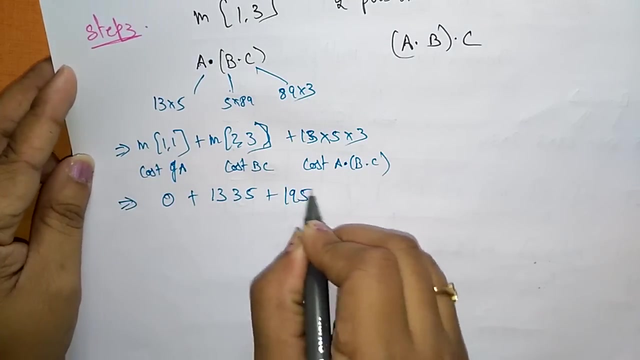 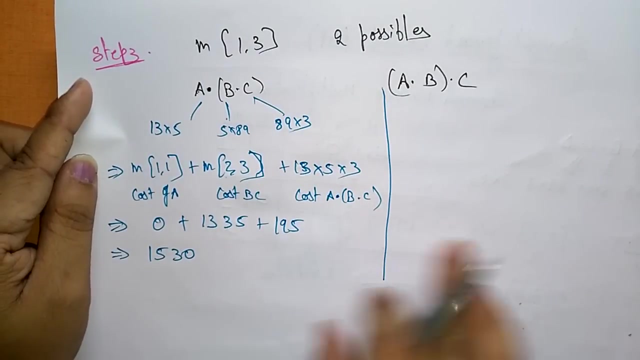 already calculated: m of 2, 3 is 13, 035, so 13, 035 plus so 13 into 5, into 3 is 195, so final the answer is 1530. so now we have to find the least possible in these two matrices. so for this m of 1, 3 there 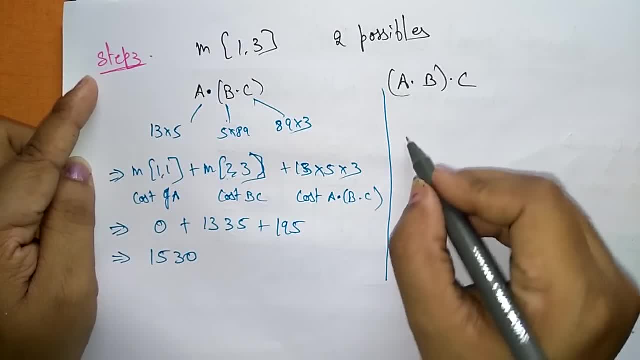 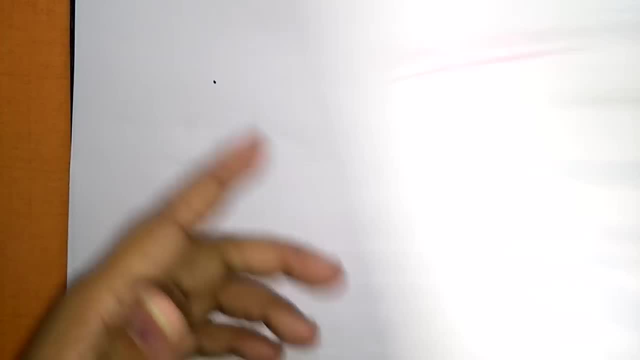 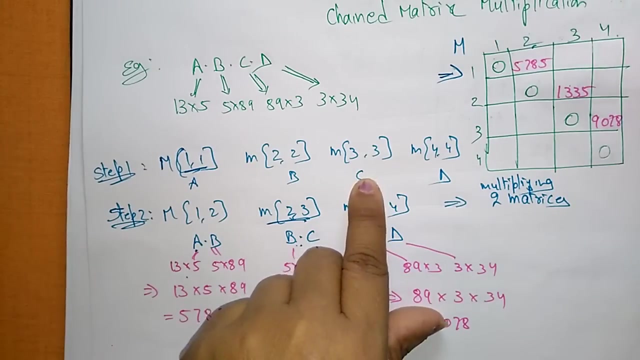 are two possibilities. so for this m of a dot b means what is the value of a dot b, a dot b, m of 1 comma 2. so that is m of 1 comma 2 and the c means what is c, c is m of 3 comma 3. 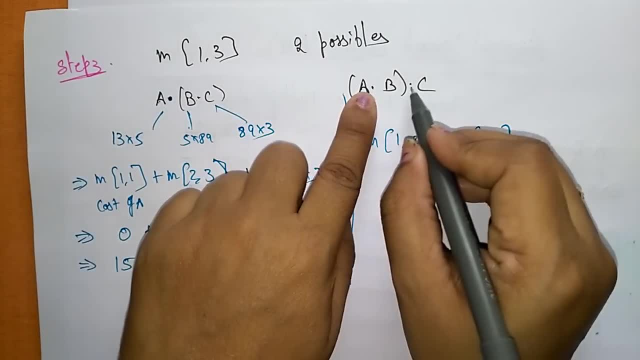 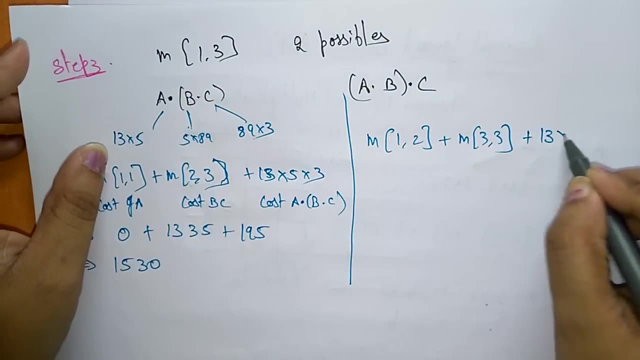 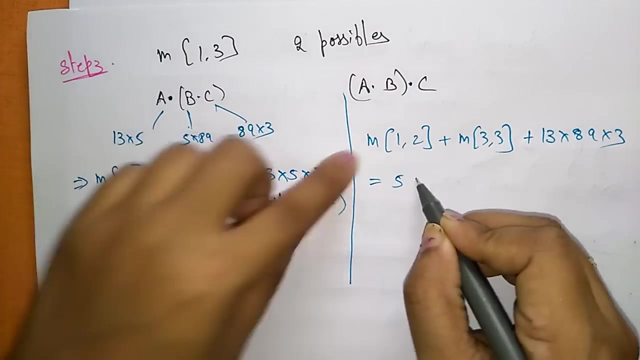 c is m of 3 comma 3 and the multiplication a dot b is: cost is over c, cost is over. now the combination of these two, cost is plus 13 into 89 into 3, so 13 into 89 into 3. so m of 1 comma 2 is 5785. we already calculated. 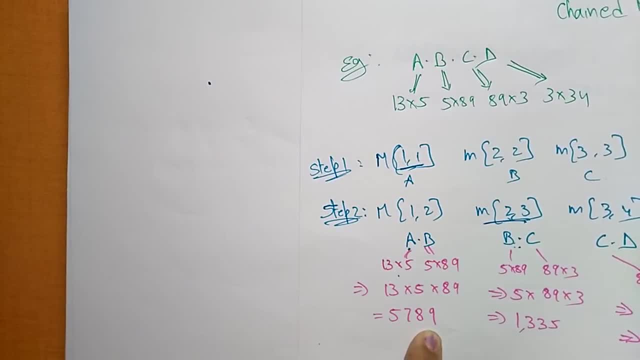 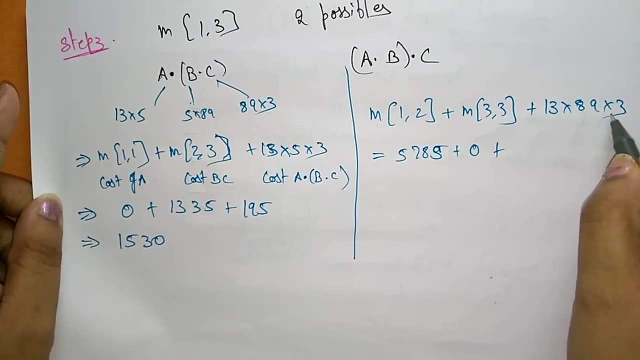 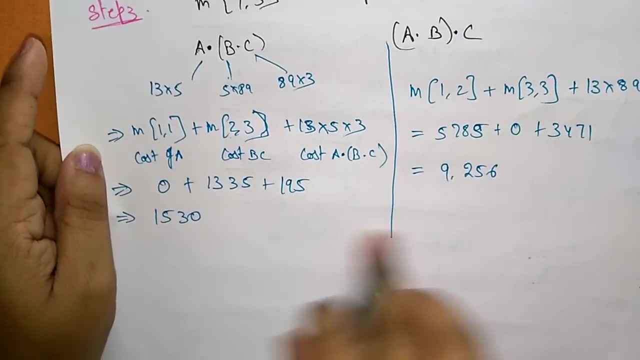 m of 1 comma 2 is 5789 and m of 3 comma 3, that is, the size, is 0 plus 0. so if you multiply this we will get 3471 and the final answer is 9256. so in these two values what is the minimum value? 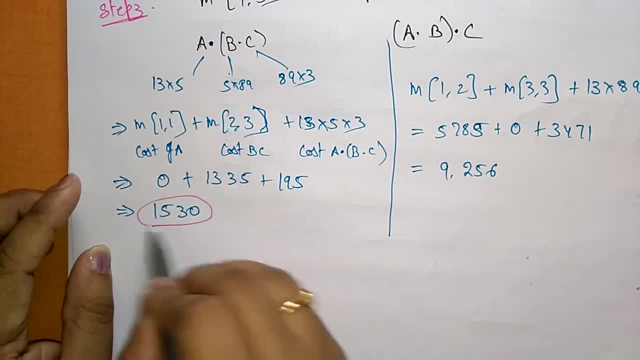 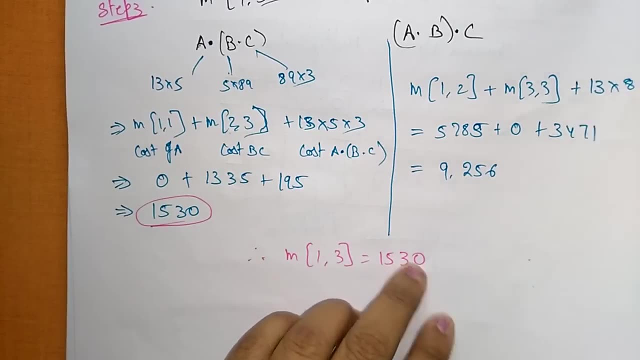 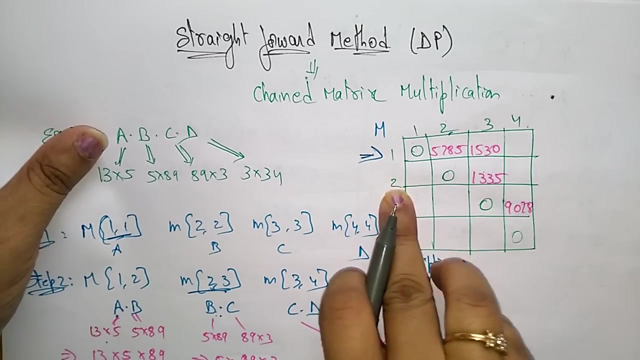 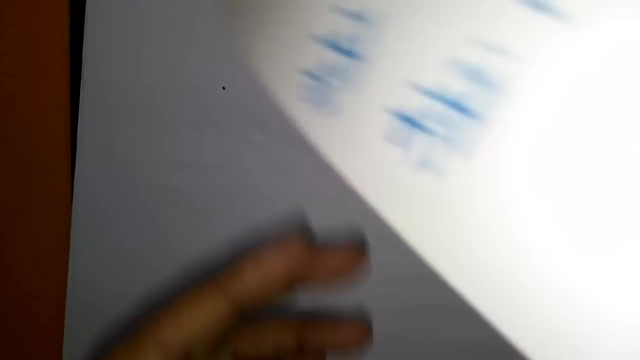 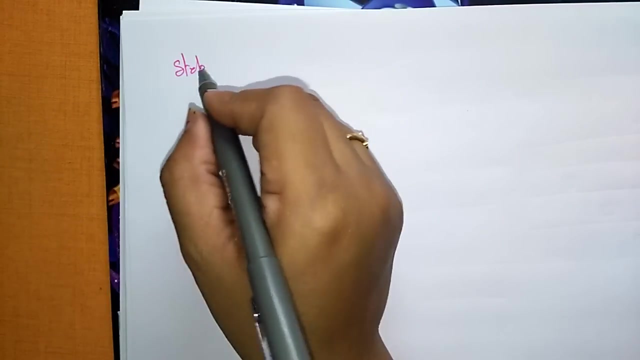 so this is the minimum. so finally, m of 1 comma 3 is 15030, so that you have to write here: m of 1 comma 3 is 15030. now i have to find out m of 2 comma 4. so let me take that next step, so the step uh 4. in the step 4 i have to find out m of 2 comma 4. 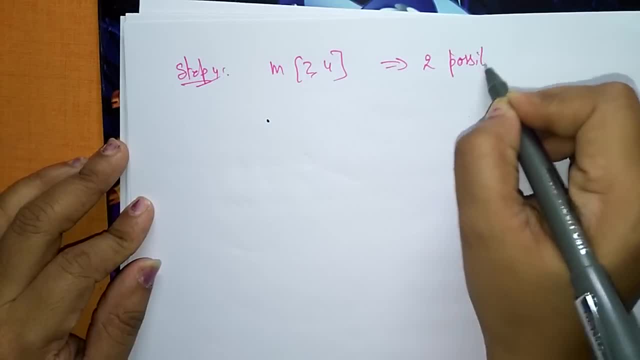 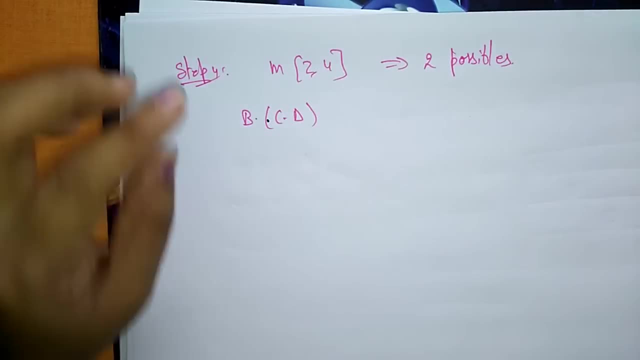 so for this also two possible multiplication is there. so that is 2. 2 comma 4 means that is b, dot c, dot d. so here just i'm one multiplication is over now i'm just doing the two multiplications. so i'm just doing the two multiplications. so i'm just doing the two multiplications. 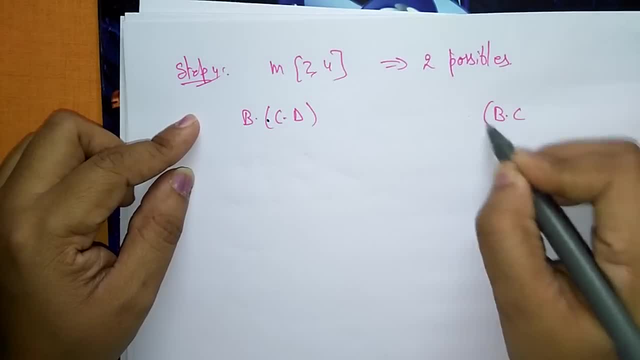 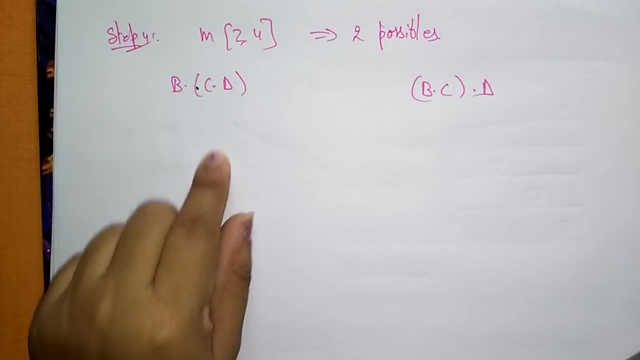 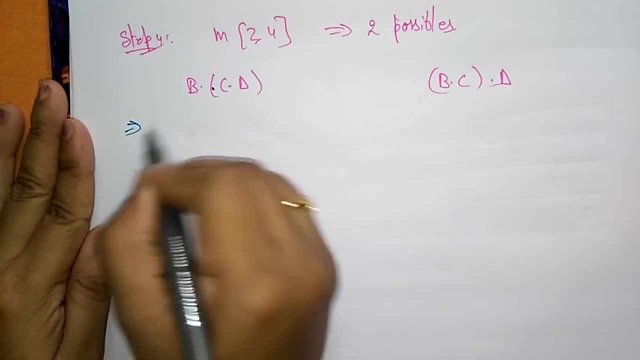 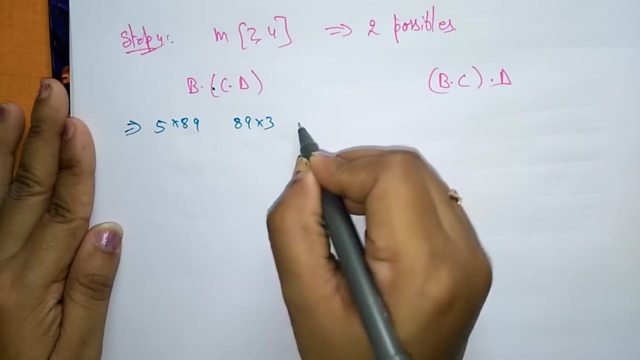 and b, dot c, dot d, or else b, dot c, dot d. you can multiply like this or this, but when you take this sequence, what is the cost of multiplying and what is the sequence for this cost of multiplying? now let us take this: b means 5 by 89, dot c means 89 by 3 and d means 3 by 34. so from this, 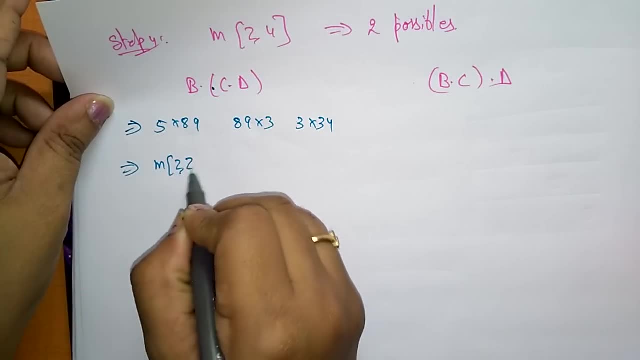 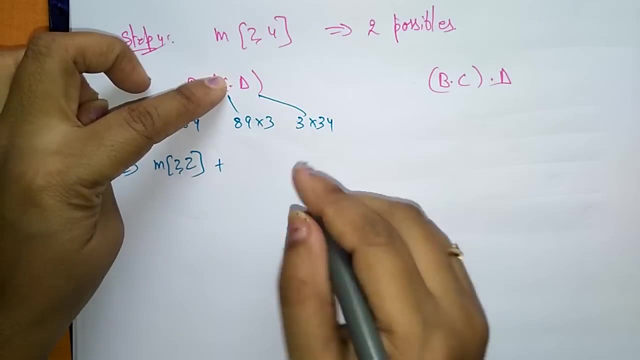 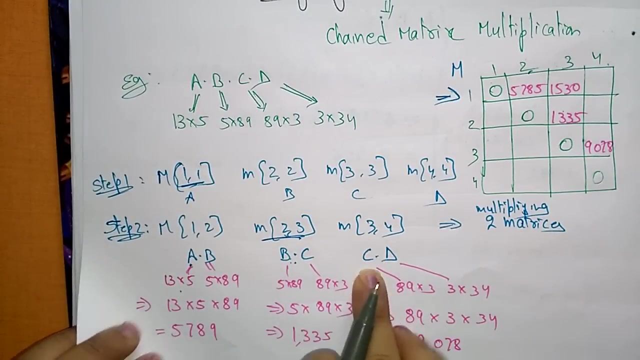 b is already is there, that is m of 2 comma 2 is b. so m of b is 2 comma 2, plus c dot d means m of 3 comma 4. so already i calculated c dot d is 3 comma 4. so plus m of 3 comma 4 and the cost of this complete. 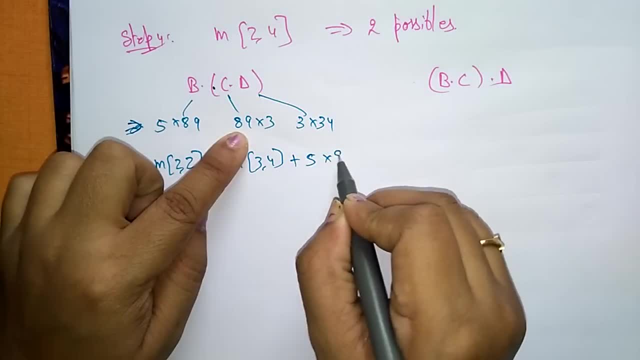 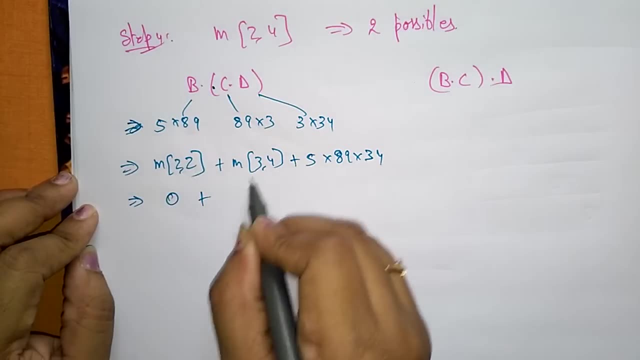 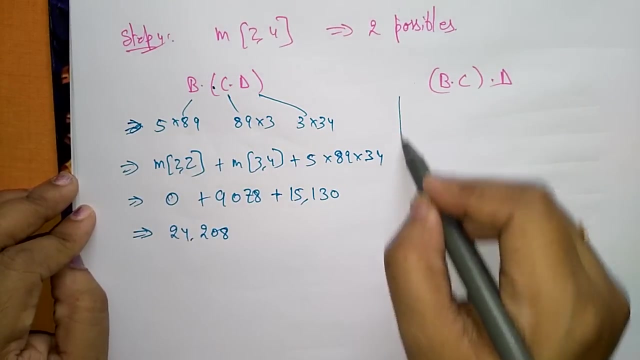 matrix is 5 by 89, by 3, 34, so so finally, m of 2 comma 2 is 0, 3 comma 4 is 9078, already calculated, and this value is 15130. so the final answer is 24208 multiplications are required, and for this c 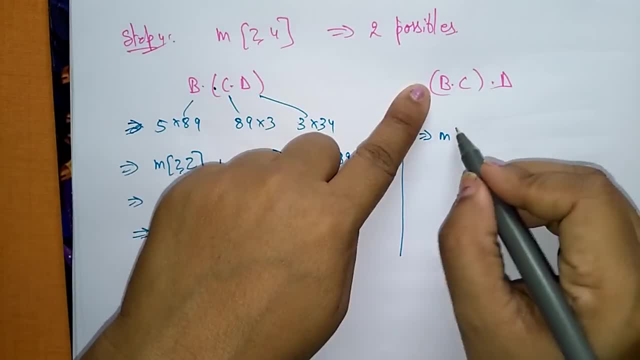 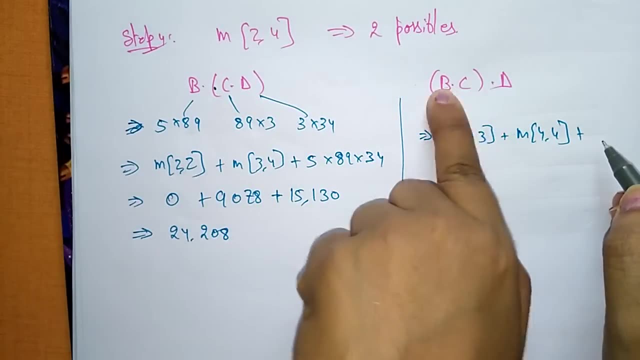 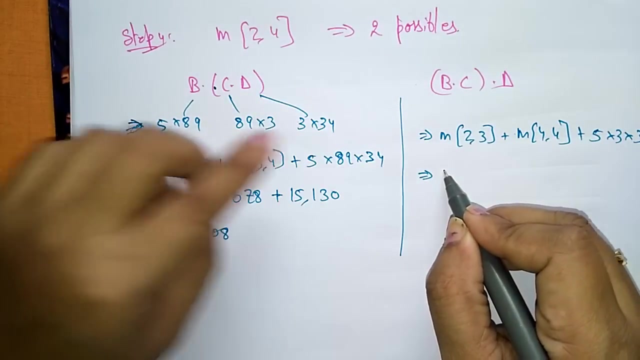 m of b dot, c means m of 2 comma 3 and d means m of 4 comma 4 plus. and the cost of multiplying this complete equation is 5 by 3 by 34, so that is, the value of m of 2 comma 3 is 13,035, 1335 plus. 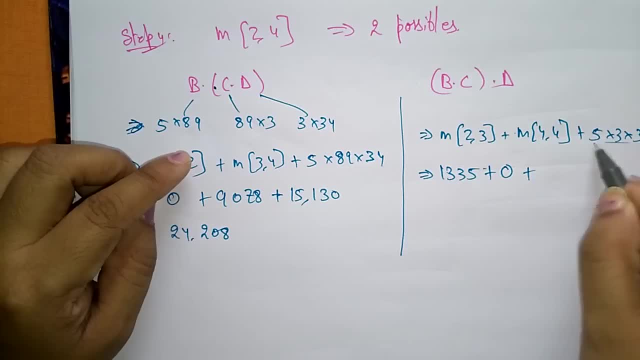 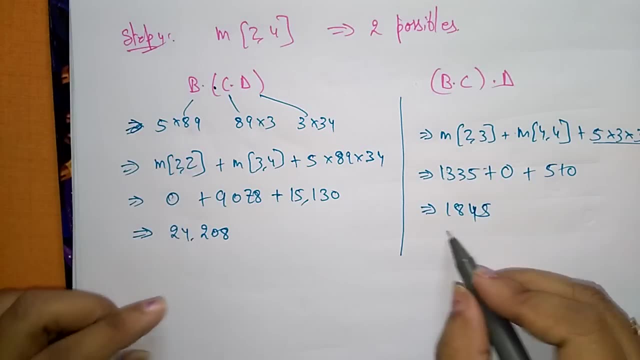 m of 4 comma 4 is 0 and the value of this multiplication is 510. so final answer is 1845. so in this, what is the minimum value? so this is the minimum value. so just write: m of 2 comma 4 is. 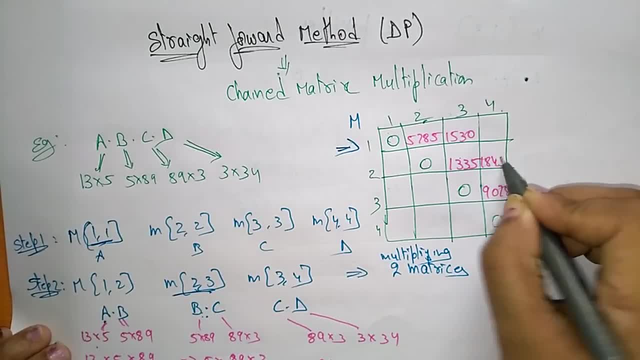 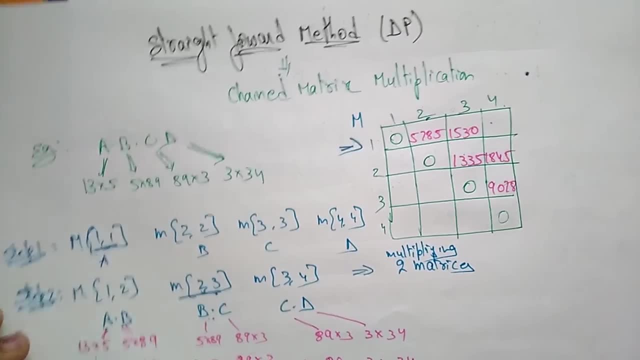 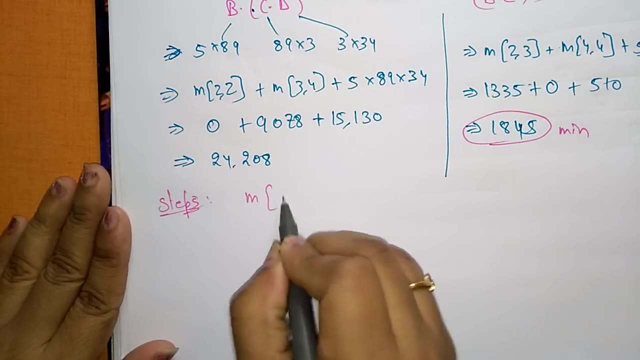 m of 2 comma 4 is 1845, 1845.. Now I have to find out m of 1 comma 4.. So for this I will apply directly the formula. So let me apply formula for this Step 5, that is, m of 1 comma 4.. 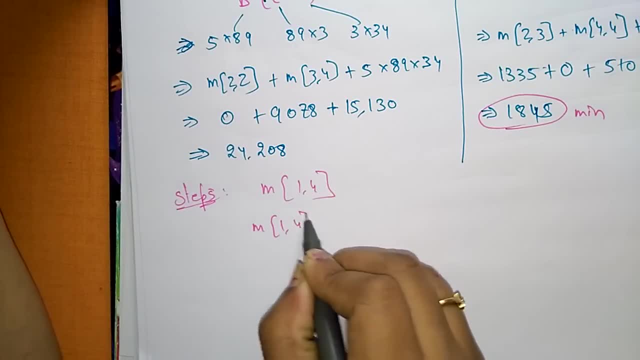 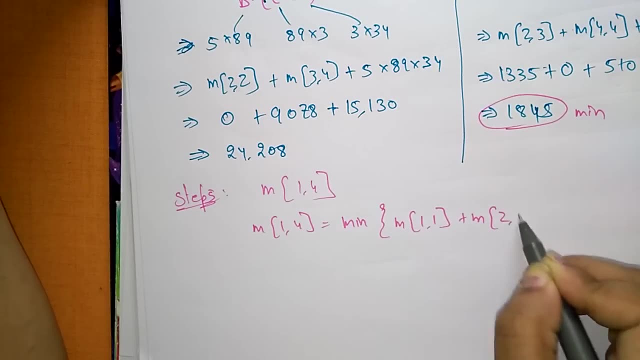 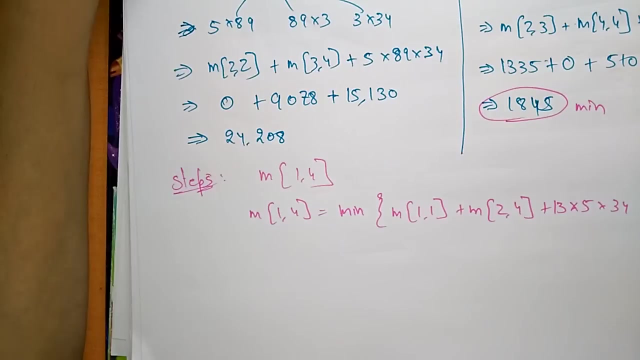 So let us take the formula: m of 1 comma 4 is equal to minimum of m of 1 comma 1 plus m of 2 comma 4 plus 13 by 5 by 34.. Okay, Comma m of 1 comma 2 plus m of 3 comma 4. 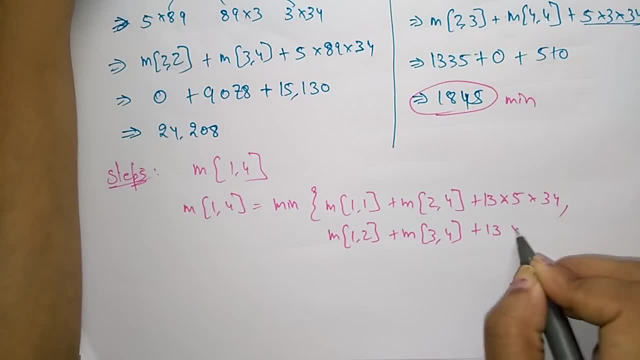 plus 13 by 89 into 34 comma. m of 1 comma 3, plus m of 4 comma 4, plus 13 by 89 into 34.. 13 by 3 into 34.. So total you are having 3 sequences. 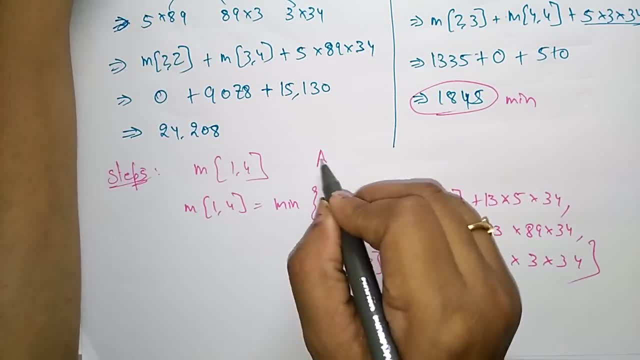 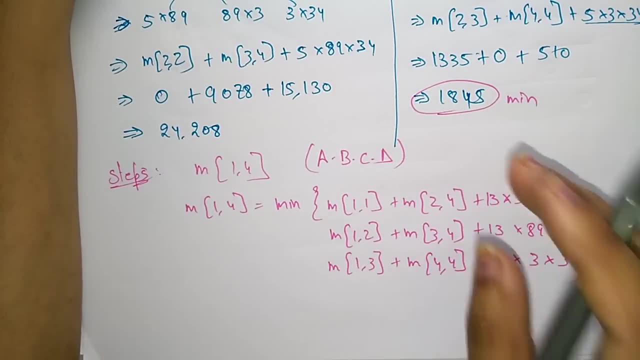 So if you want to multiply 4 matrix, 1 to 4, that is a dot b, dot c, dot d. So if you want to multiply this 4 matrices, you need 3 sequences. Okay, So the 3 sequences are a dot b, dot d, c, or a dot b, dot c, dot d or else. 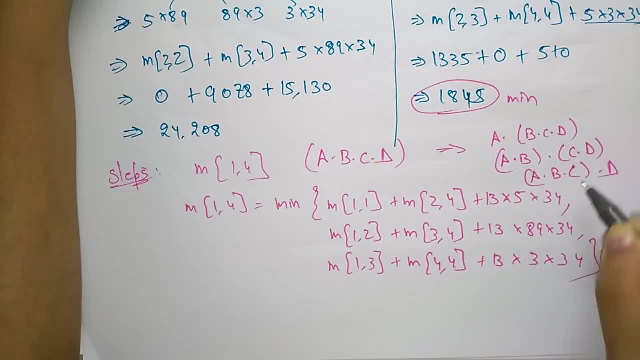 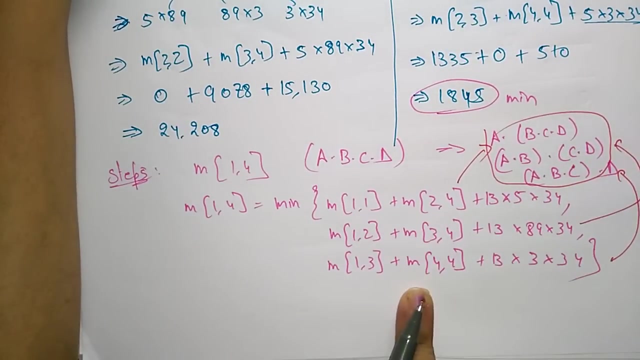 a, dot b, dot c, dot d, So whatever I have entered here. So this is the first sequence, and this is the second sequence, and this is the third sequence. So these 3 sequences I have written like this. So for each sequence this is the cost of multiplying. 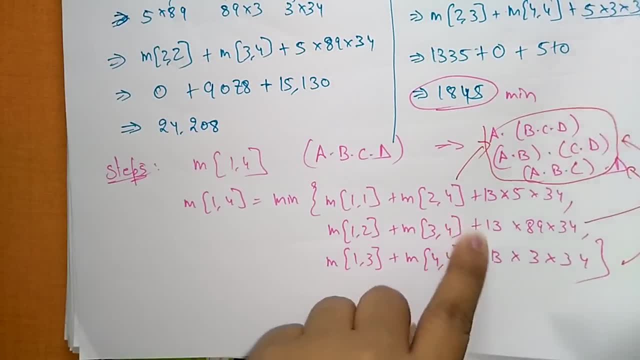 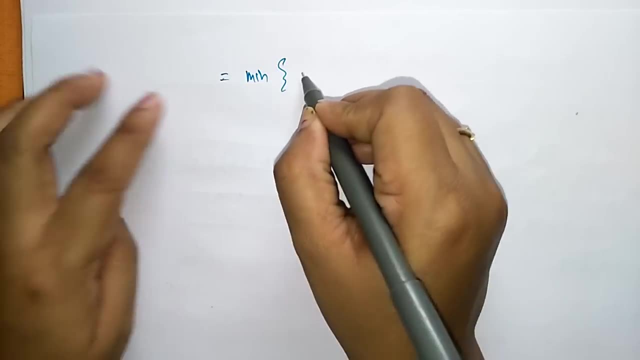 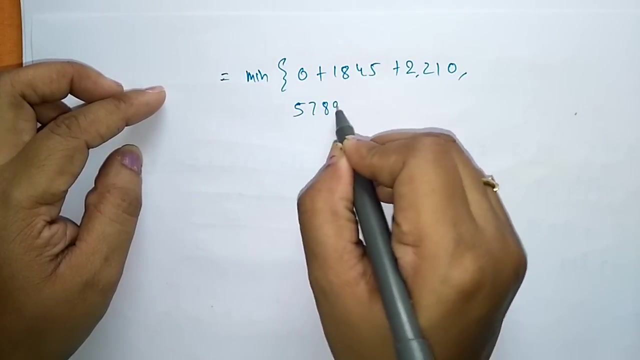 the matrices. So, and the final, if you calculate this thing, everything so, you will get minimum of zero plus one, eight, five, five plus two thousand two, ten comma, five thousand seven, eighty five plus eight, zero, seven, nine zero, seven, eight plus thirty nine thousand three thirty eight. 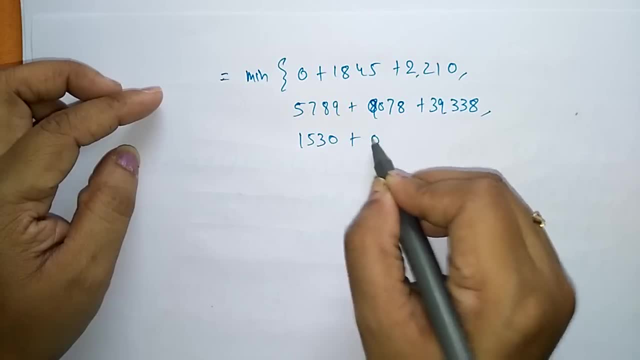 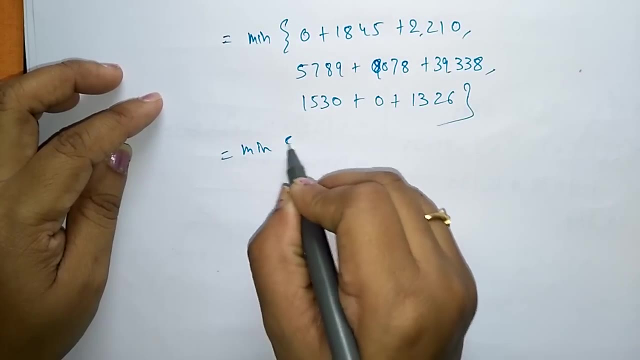 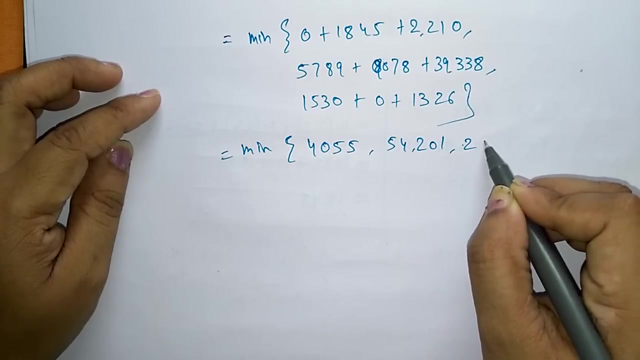 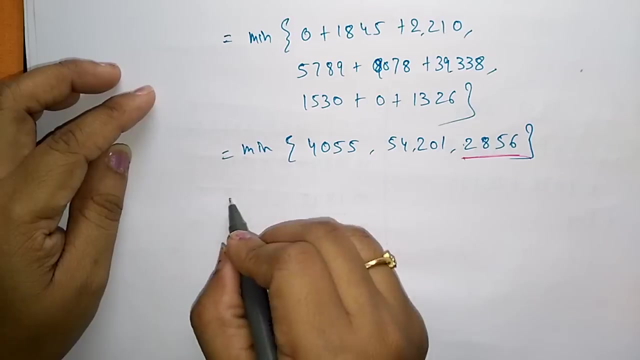 comma fifteen hundred and thirty plus zero, plus one thousand three twenty six. Okay, So if you add all those things, the minimum of four thousand fifty five comma, fifty four thousand two, 1 comma 28,056.. So from all this, what is the minimum value? So the minimum value is: 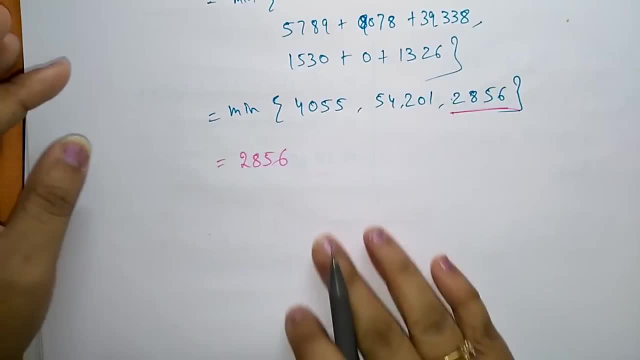 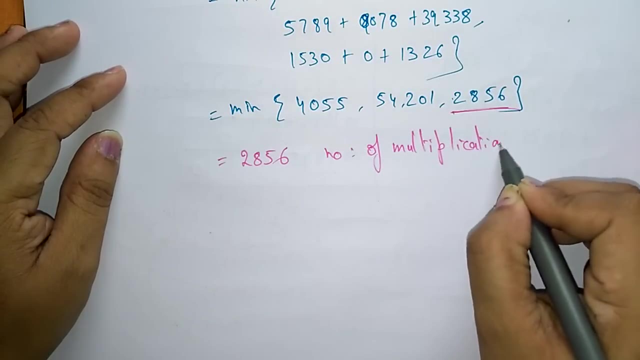 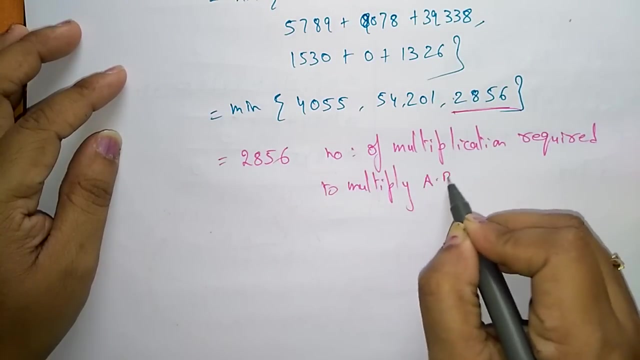 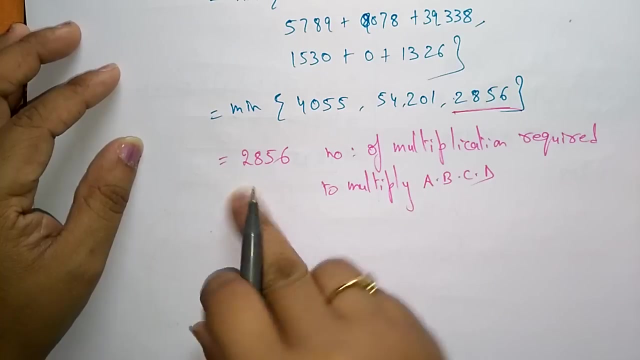 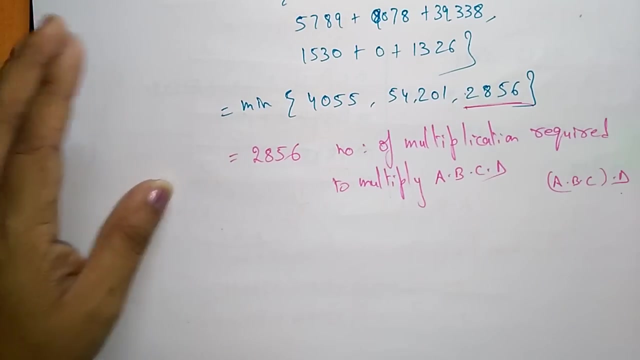 2,856.. So the total number of multiplications, number of multiplications required to multiply a dot b, dot c, dot d, is 2,856.. So that is a sequence. the sequence that you require to multiply this is a dot b, dot c into d. Okay, So let me write the formula for this. 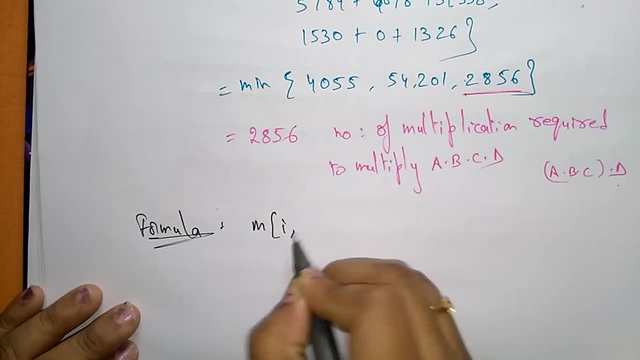 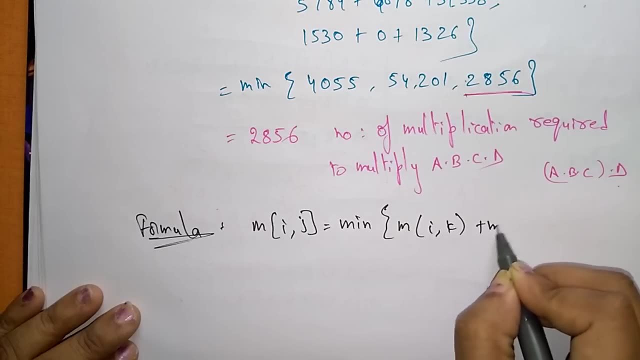 So the apply. I applied the formula like: m of i comma j is equal to minimum of m of i comma k plus m of k minus k plus 1 comma j plus d of i minus 1 into d of k, into d of. 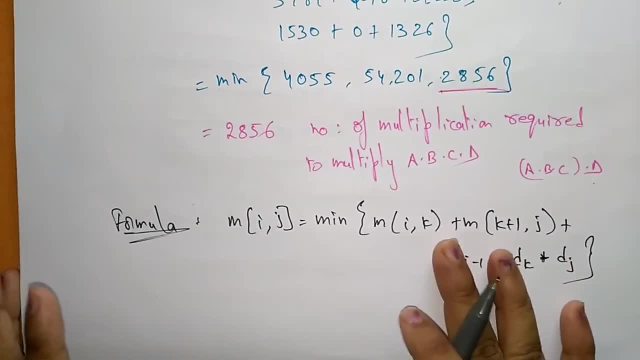 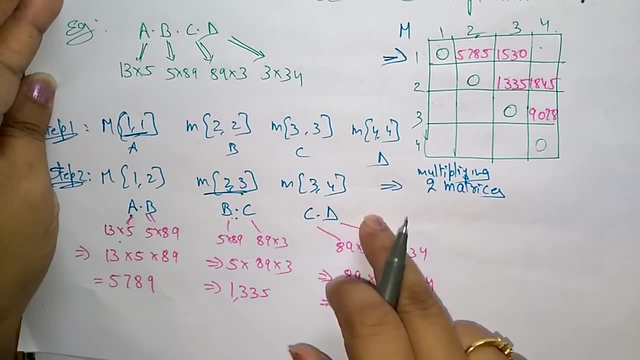 j. So this is a formula, So don't be confused about this formula. just, whatever the procedure I have followed to calculate all those things, So these values, whatever the procedures I have taken to calculate. So this is the cost of multiplying only a maximum. 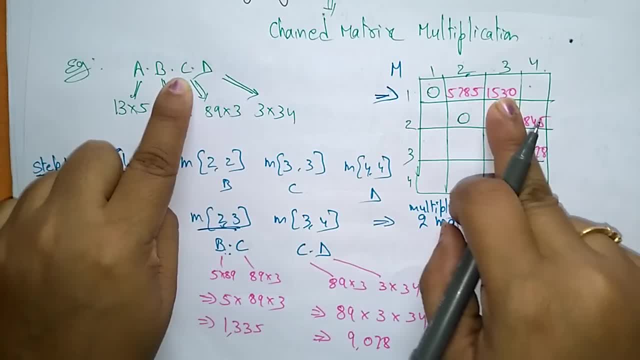 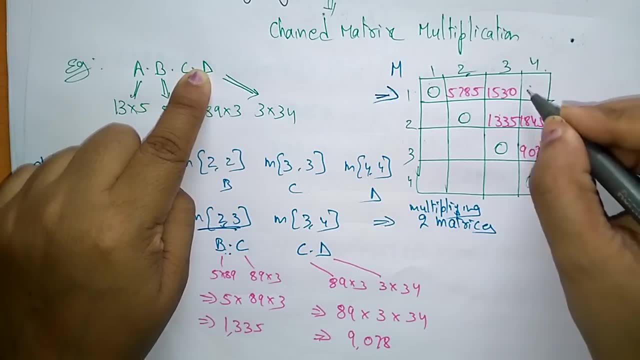 So this is the cost of multiplying a by b matrix and a into b into c, the three matrices, and the final is a into b, into c, into d, So that you get is 2,856.. Okay, So we want.